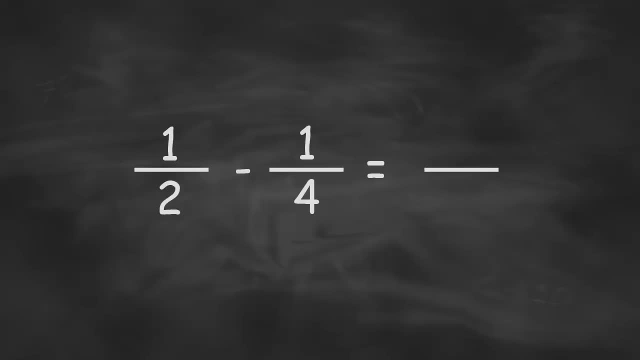 So that's a pretty easy example. This next example seems a little harder, but it's pretty easy as well. So we have 1 half minus 1 quarter. Now we can't just subtract 1 quarter from 1 half, because they're not the same thing. 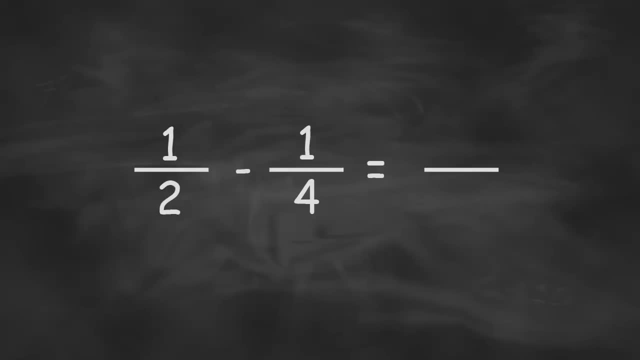 It's like subtracting apples from oranges, But we can see in this example that it would be pretty easy to turn our half into quarters. So in this example we're going to take our 1 half and multiply the top and bottom by 2.. 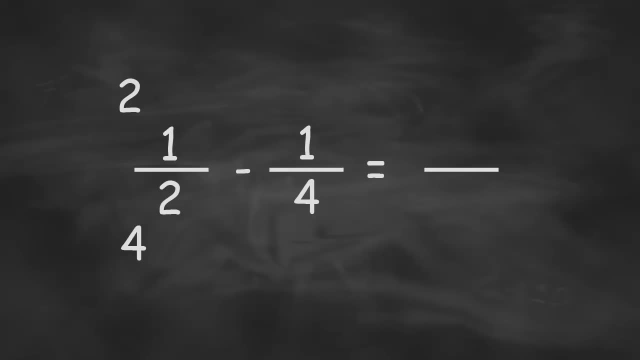 So we're going to get 2 on the top and 4 on the bottom. So we took 1 half and now turned it into 2 quarters. Now you have 2 quarters minus 1 quarter. Since those are the same denominator, we can just subtract 2 from 1,. 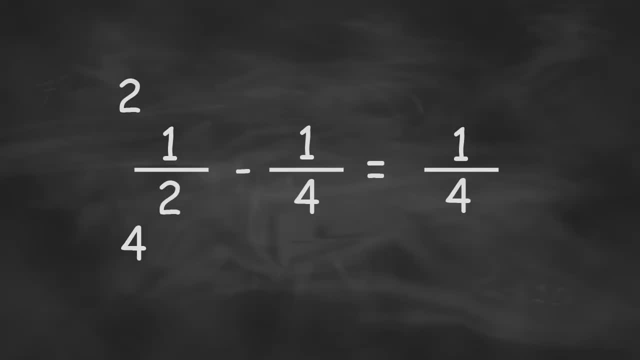 leaving us with 1 quarter. Now here's where it gets more complicated. In this example, we have different denominators and we can't easily make one denominator match the other. So here's where our handy trick comes into play. 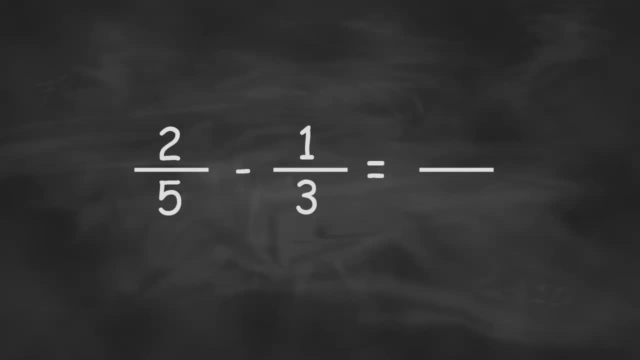 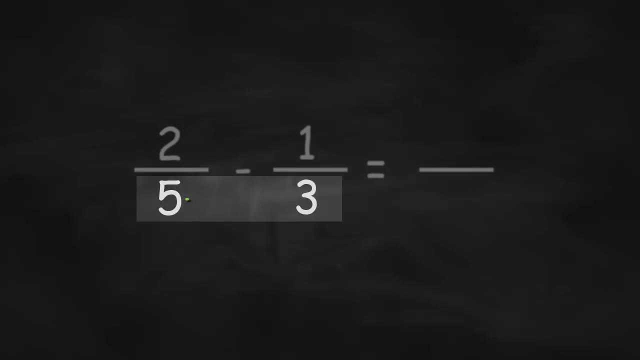 You can use this for any fraction, subtraction problem or addition problem, for that matter. So all we have to do here is multiply the bottom numbers. So in this case, we take 5 times 3, and we get 15.. 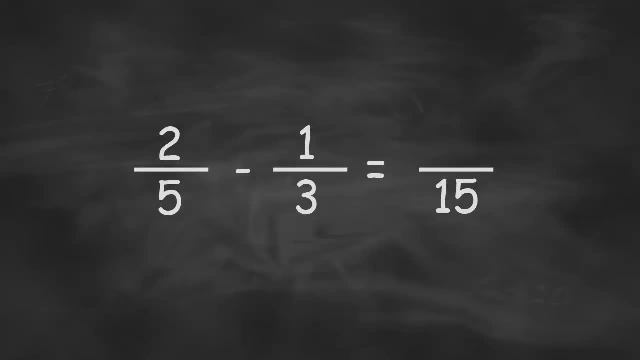 That's going to become our denominator, That's going to be the denominator of our answer. Then we start in the top left-hand corner and we multiply diagonally with the other denominator. So 2 times 3 gives us 6.. 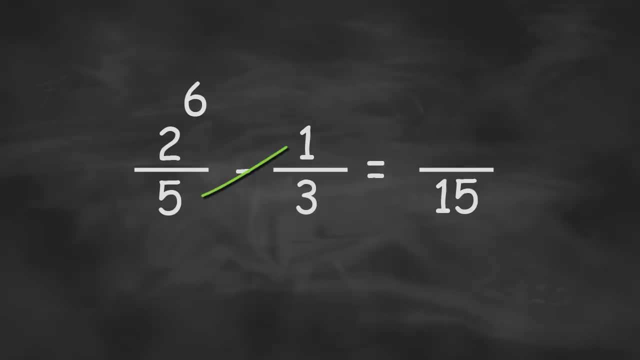 Then we take our other top number, our other numerator, 1, and multiply diagonally with the 5, and we get 5.. Now we can take our 6 and our 5,, just subtract those following the symbol in the middle of the problem. 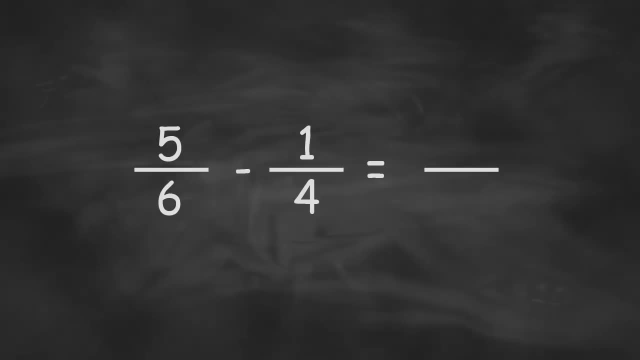 and we get 1- 15th. Now, it's not always that easy. We can use this same method, but just make sure that when you get your answer, it's in its simplest form. Take, for example, 5, 6 minus 1 quarter.